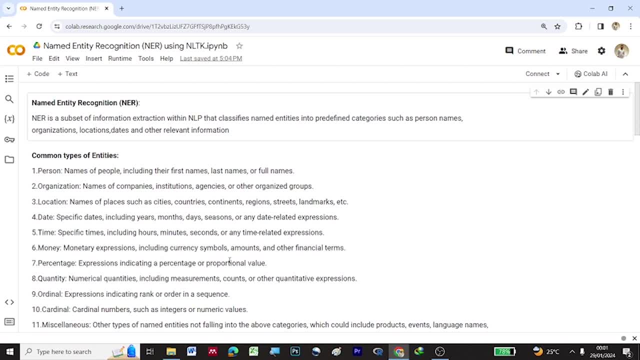 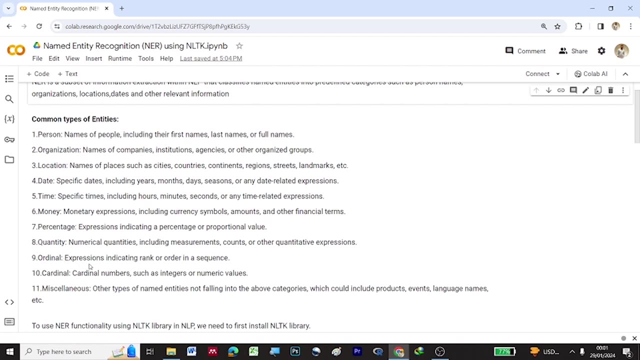 Under money, you will have monetary expressions, including currency symbols. amounts, percentage: You will have expressions indicating a percentage or proportional value. Under quantity, you will have numerical quantities, including measurements, counts or other quantitative expressions. ordinal expressions indicating rank or order in a sequence. cardinal numbers, such as integers. 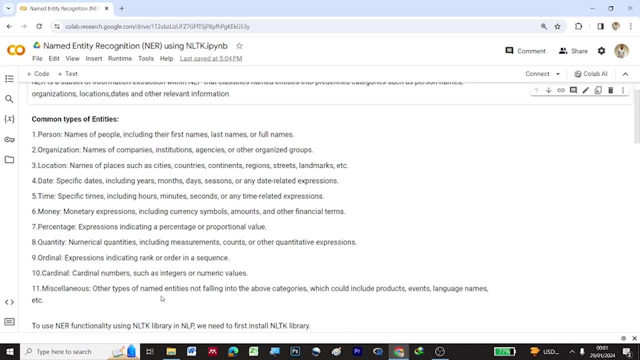 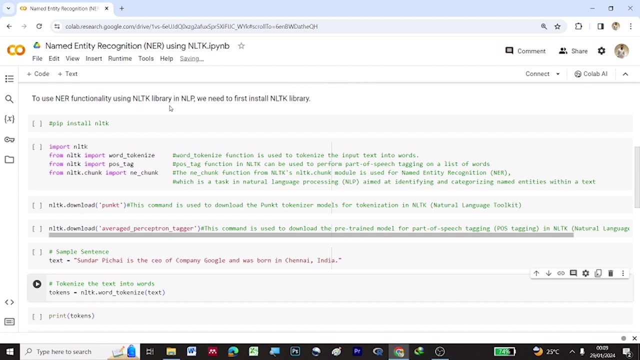 or numerical numbers, miscellaneous other types of named entities not falling into the above categories, Which could include products, events, language names, etc. Now let us come to the coding part. To use the NER functionality using NLTK library in NLP. 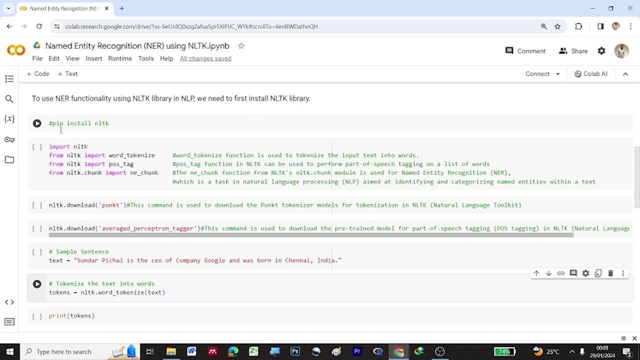 we need to first install an NLTK library. So let us install this by using pip: install NLTK. So once we have installed, we will import NLTK. Since this NER, named entity recognition, needs some pre-processing, We are supposed to do tokenization, Then we are supposed to do POS tagging, Then at 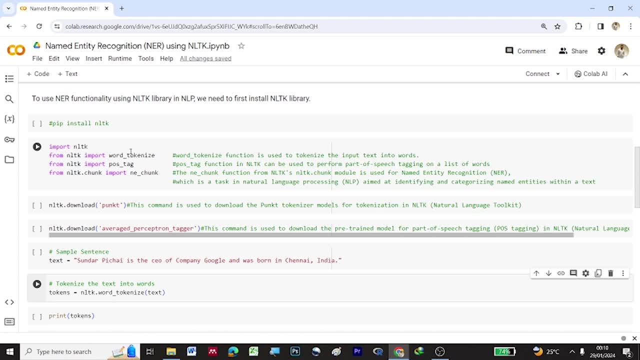 later stage you will be doing named entity recognition. So for that, since tokenization process is involved, so I am importing word tokenize from NLTK. Then, since we have to use POS tagging, so I am importing POS underscore tag function And later on, since I have to, 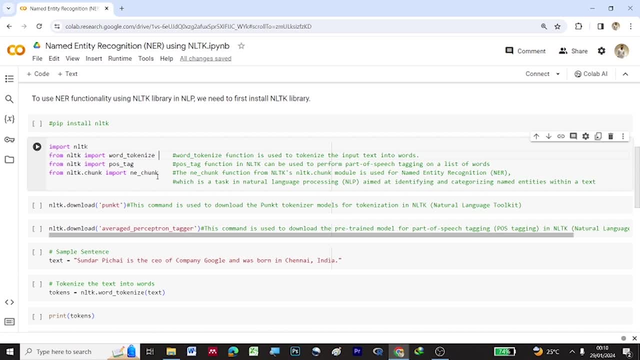 do the named entity recognition. so I am going to use any underscore chunk. So we know what is word tokenize. Word tokenize is nothing, but it's a function which is used to tokenize the input text into words. And POS underscore tag is a function in NLTK that can be used to perform parts of speech. 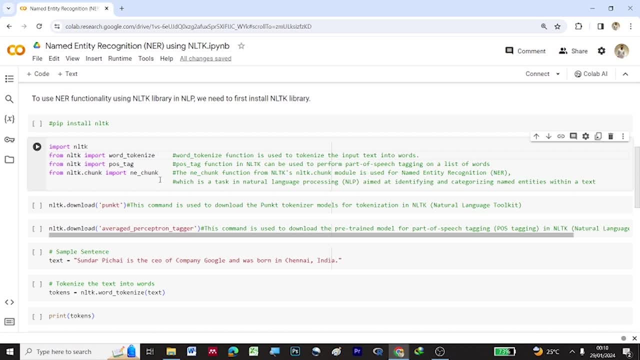 tagging on a list of words: NE. underscore chunk- that is named entity. underscore chunk function from NLTK- that is NLTK dot chunk. So it means it comes from here, from NLTK. dot chunk Model is used for named entity recognition with the task in NLP. 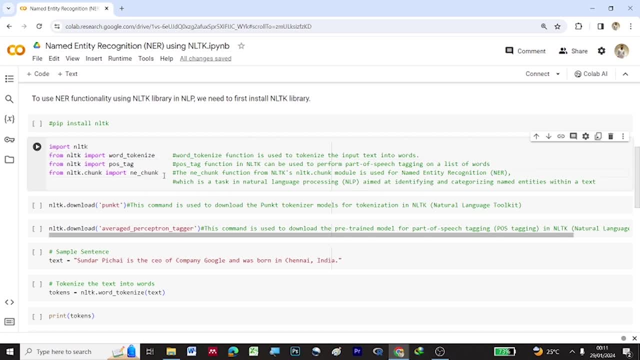 identifying and categorizing named entities within a text. Let us import all this, Since we are involving tokenization process, so definitely we have to download punkkt. So this command is used to download the punkkt tokenizer models for tokenization in NLTK. 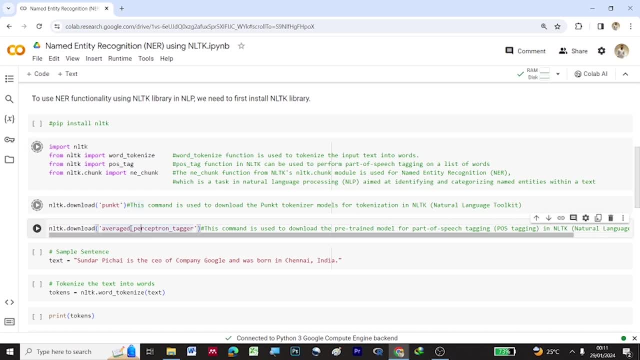 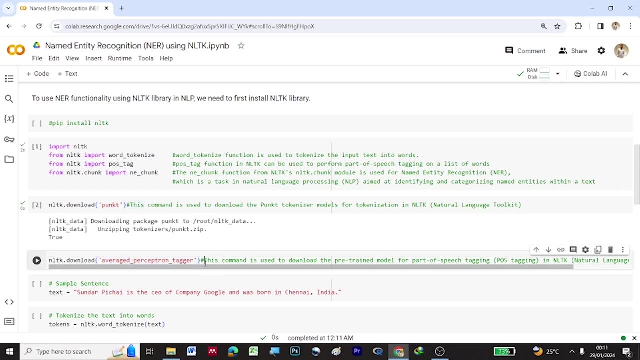 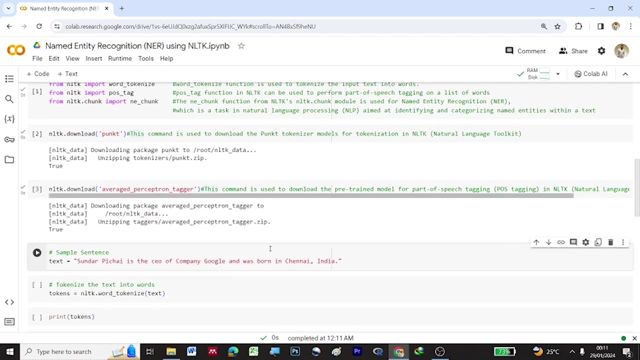 So once that is installed, we'll be installing average underscore, perceptron, underscore tagger, since we want to perform POS tagging, So we will download this also. This command is used to download the pre-trained model for parts of speech tagging. Okay, so once these functions are downloaded now we will provide a sample. 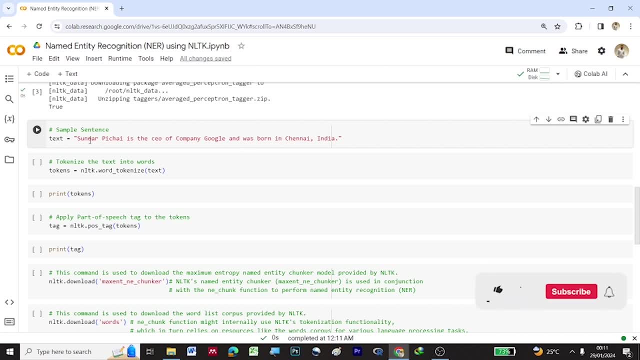 sentence. So here I am providing a sentence, as Sundar Pichai is the CEO of company Google and was born in Chennai, India, And I am storing this sentence into the variable called text. Okay, so now I have to tokenize this. 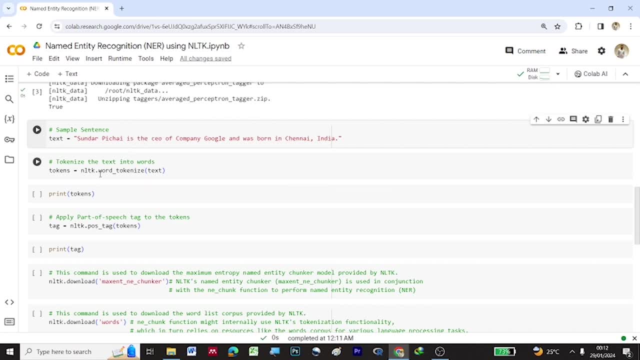 A particular sentence. So I'm applying NLTK dot, word underscore, tokenize, And I'm giving this sentence as the input to this. Okay, so let me execute this text variable And I'm storing that the output of this will be stored under tokens. Okay, so let me print the tokens And you can see. 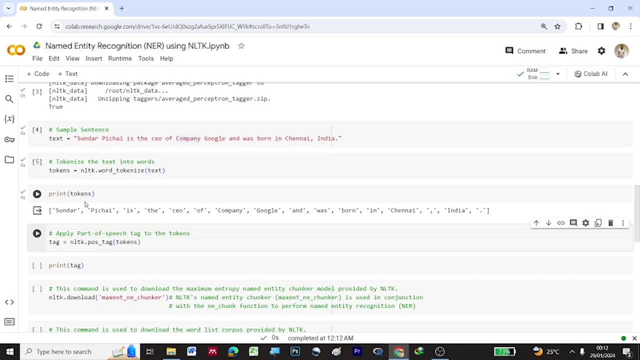 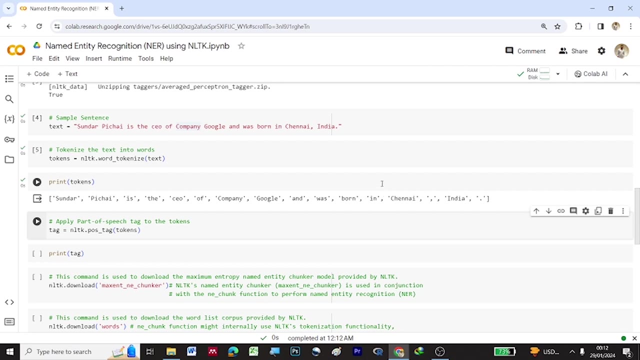 each word in the particular sentence has been broken down as individual words. Sundar Pichai is the CEO of. everything has been broken down. even the comma has been breakdown. Okay, so once we have done this word tokenized, we have to correspondingly apply POS tagging, that is. 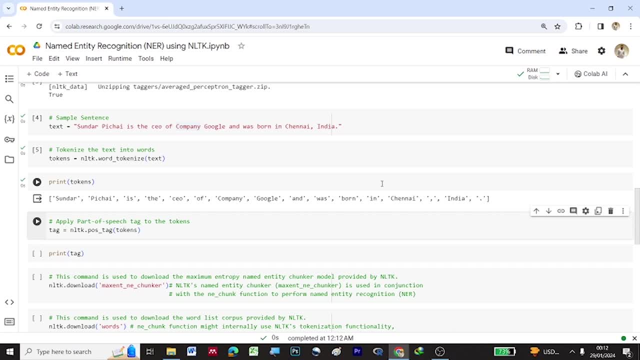 for each, correspondingly each words, you will have their corresponding grammatical categories, like noun, verb, adjective. Okay, so I'm going to apply NLTK dot POS underscore tag, taking this tokens and applying applying that as the input to towards this and I'm storing that. 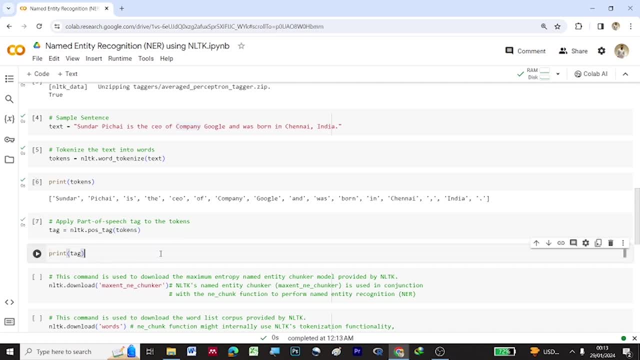 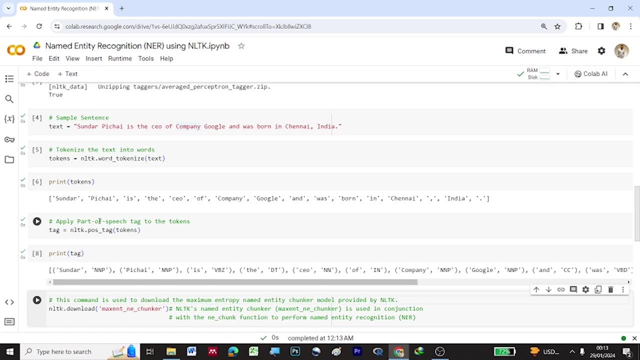 under tag. So let me print the tag. Okay, so correspondingly, the grammatical categories of each of the words has been given here. like Sundar, it belongs to NNP. Pichai belongs to NNP. Similarly, the belongs to determiner. Okay, so we know what is NNP. 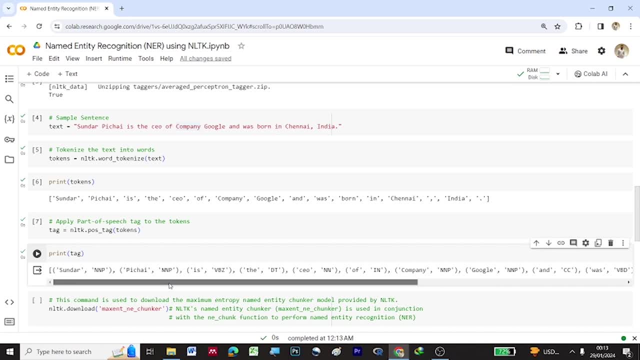 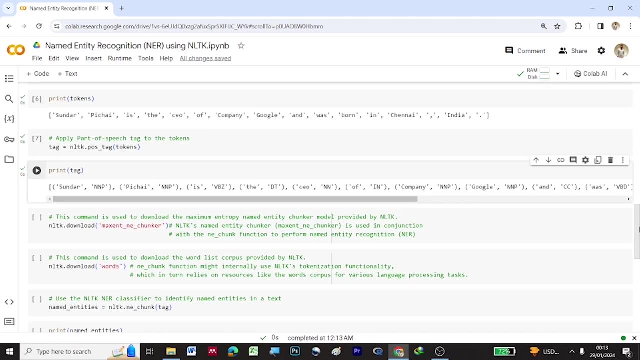 and we have seen in the previous video, so you can refer the previous video for POS tagging. Okay. so let me come down a little bit. So once we have done the tokenization process and we have also completed the POS tagging, Okay, so now we have to import the necessary functions for doing. 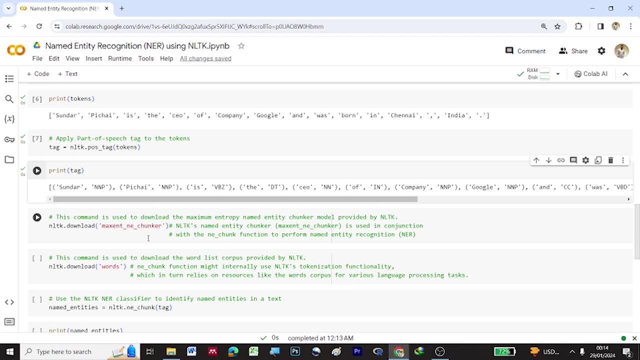 the named entity or for finding the name entity recognition. So here we'll be importing this particular command: Max ENT underscore and N E underscore chunker. So what is this? this command is used to download the maximum entropy named entity chunker model provided by NLTK, And this NLTK is named entity. 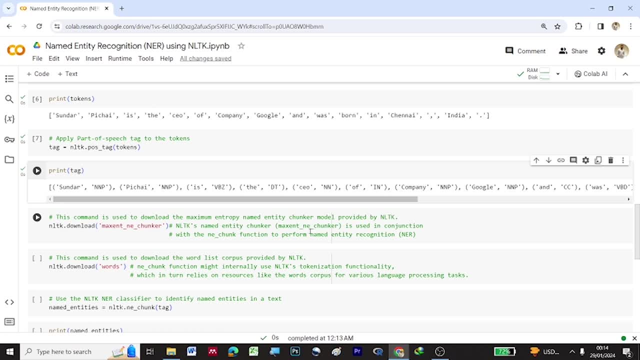 entity chunker, that is, Max ENT underscore. N E underscore chunker is used in conjunction with the N E underscore chunk function to perform named entity recognition. Okay, so this function it. it matches along with the N E underscore chunk function. Okay, since we have imported it from the starting right. 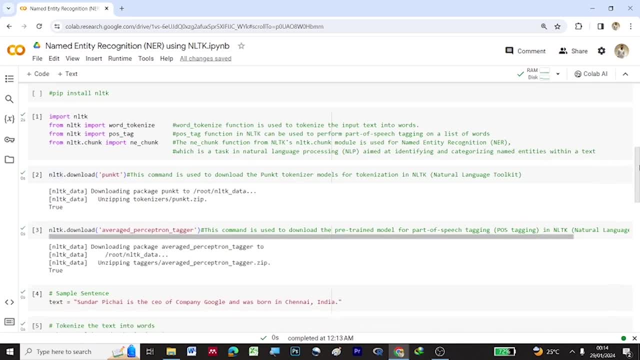 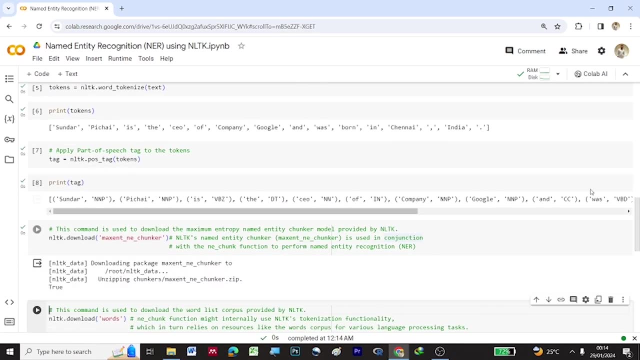 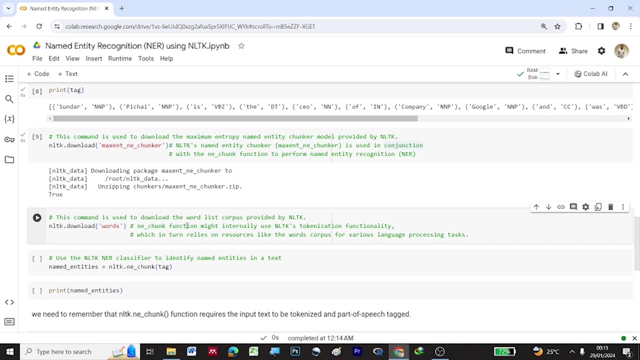 okay, so it will work along with that to give you the output of any R. Okay, so let me execute this. Okay? correspondingly, we have to also download NLTK dot download words. Okay, so this command is used to download the word list corpus. 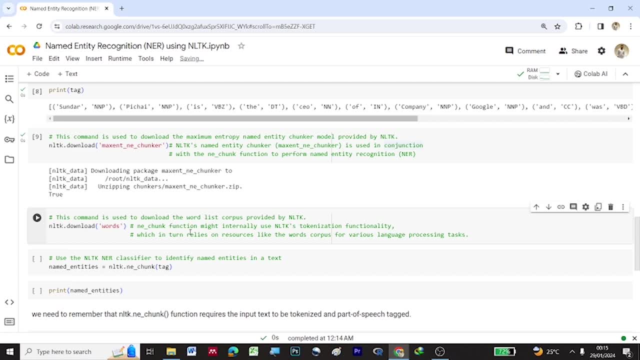 provided by NLTK. So N E underscore chunk function might internally use this NLTK tokenization functionality which in turn relays on resources like the words coppers for various languages, closing tasks. this particular function will internally use the tokenization process. Okay, So it means that tokenization functionality means we have? 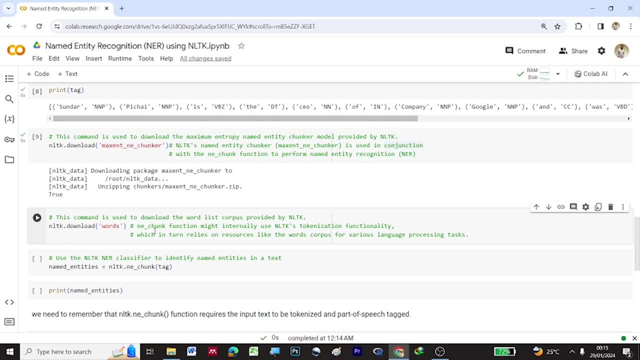 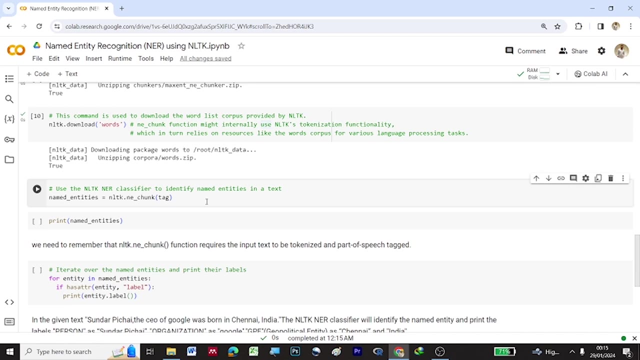 something called corpus- right word corpus. So we have to download this word corpus. Once this has been downloaded, Okay, we'll get next. we'll be. we'll be moving to find out the corresponding name entities in a particular text, so we'll use the nltk. any. 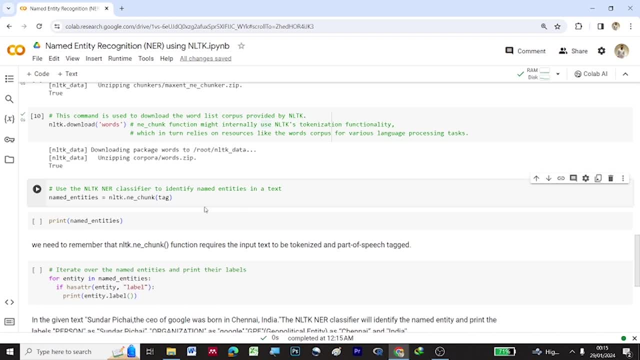 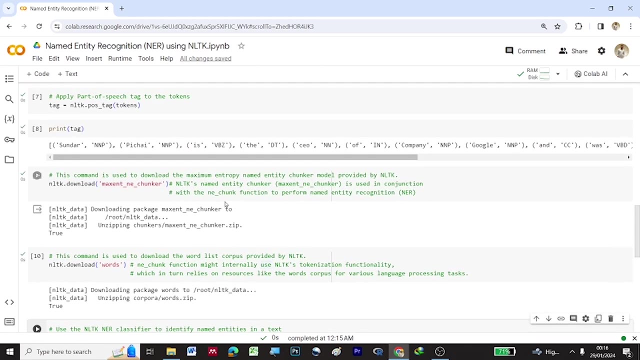 ner classifier to identify the named entities in a text. for that we'll use nltk dot, any underscore chunk, and the input to this is tag the one, what we have done, the tagging right, the corresponding grammatical categories. that particular tag will be given here. you can see here this particular. 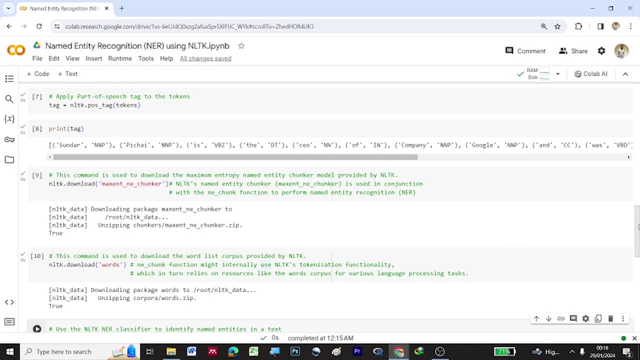 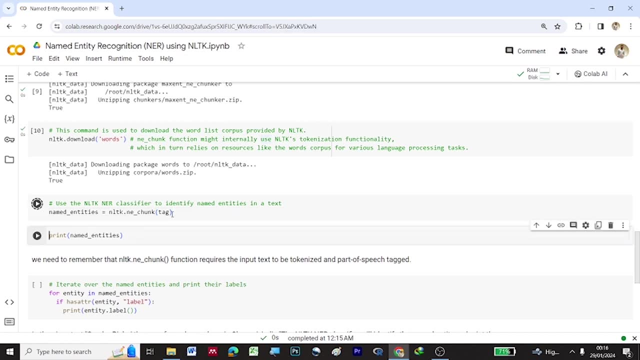 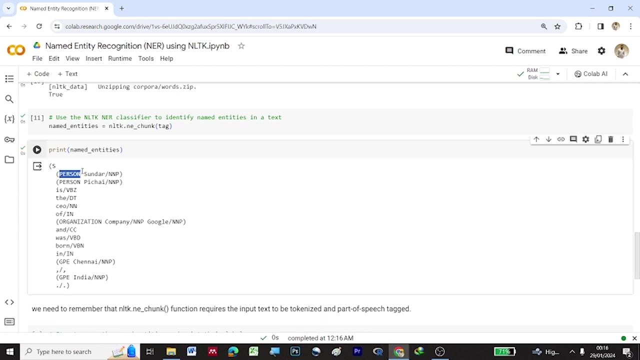 thing. okay, will be given as the input for the any underscore chunk. okay, and it will be stored under the variable named underscore entities. okay, so let us print and see what are the named entities. okay, so here we have this named entity called person. under the person, we have the name of the person. okay again. 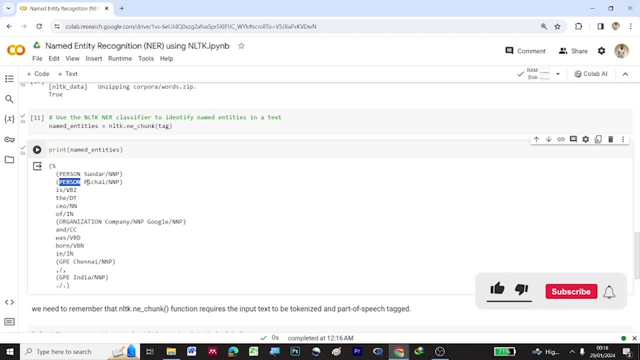 in the same. we have person and the name of the person. we have difference as pitch. i similarly we have is the ceo. okay, here again we have the. so these are not entities here. okay, so we'll be coming to the next entity. we have organization- you know that company- and google. they come under the organization. similarly, we have gp. 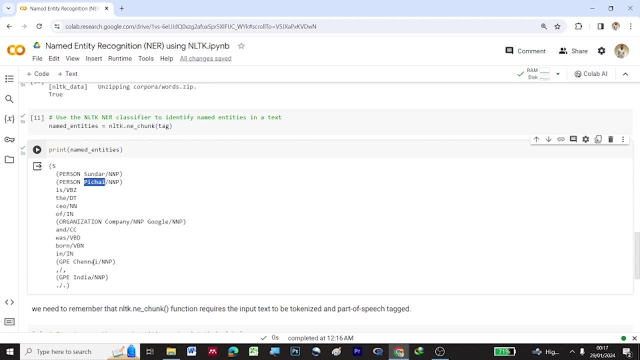 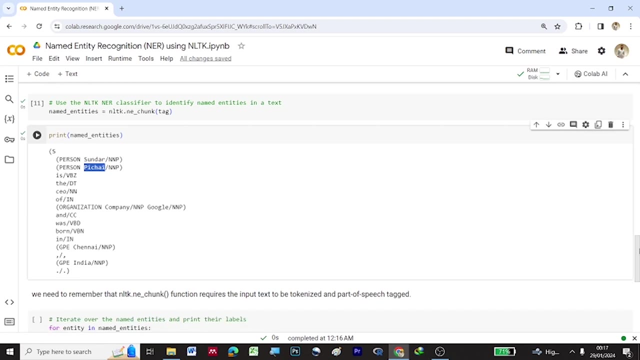 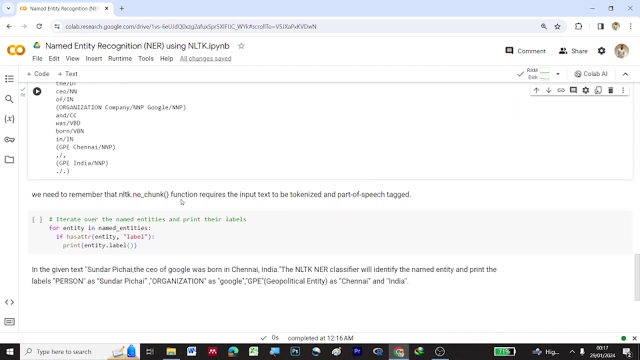 gp, gp, gpe. we have chennai and india under gp. so what is gp? gp is nothing but the geopolitical entity. okay, so here we have uh, entities like person, organization and gp. okay, so all these are the name entities here. okay, so now we need to remember that nltk dot- any underscore chunk function, requires the input text. 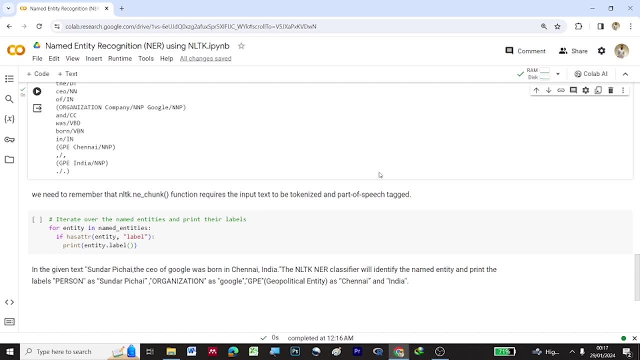 to be tokenized and a part of speech tag. okay, that is what we have studied, right? so this is like a node. you have to remember this. okay, now let us print the desired labels, like: what are the entities which we have got from the sentence? okay, so, because of the entities which we have got, we got person. 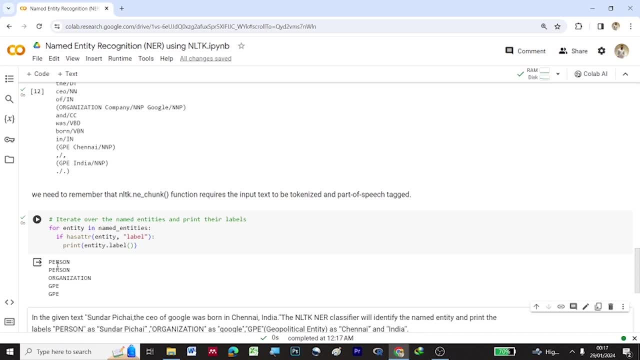 person because we we had the name right, like sundar pitchai, so sundar was identified as person name and picture was also identified as person name: Hassan, since i have got Google сitemyда right, so it was. it comes under the entity called organization. we have, we have gp, like i told you, geopolitical uh entity. geopolitical entities means like uh location are entities, like videos are located and you have to give a while, or 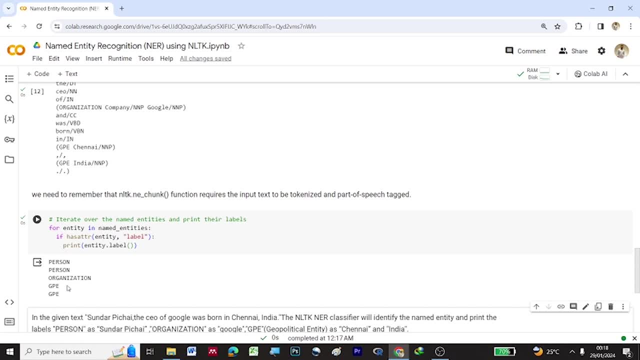 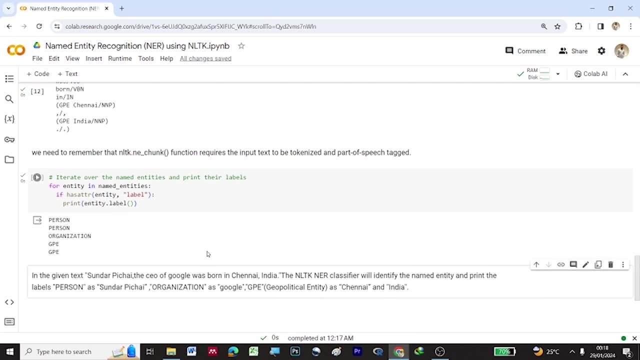 locations, right. so that's just, that's true. or, if you haven't watched the video, we will use google term, that's just like also, which is traditional locations, right, so we have chennai and india. so okay, so in the given text, in the picture, the ceo.